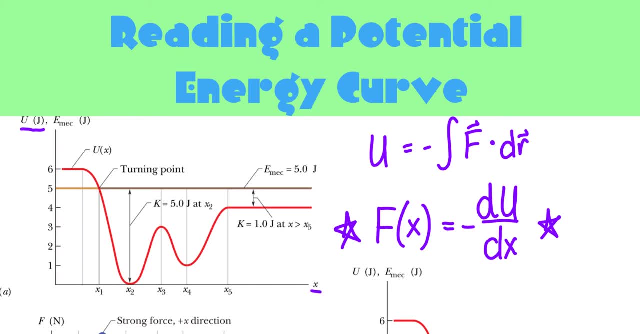 potential energy specifically versus position graph, as I do here, I can find the slope of that graph and the negative slope of that graph is equal to the force. That's one important way of using these potential energy curves. You'll also notice something that's commonly: 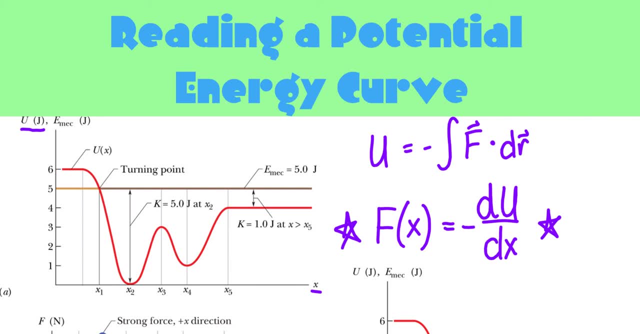 included in the equation is the energy of the force. So if I have a potential energy on a potential energy curve is a straight line that tells us about the total mechanical energy of our object. like you see here, We know that an object's total mechanical energy is a set value. 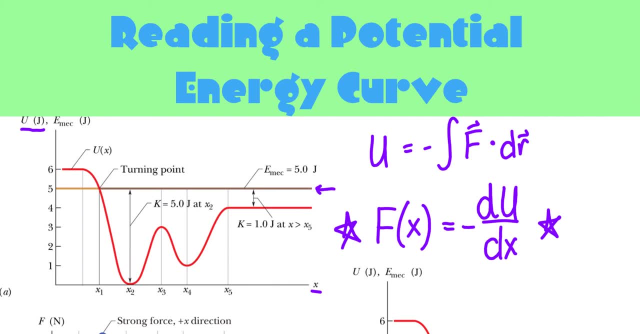 It can never magically gain energy, And if all the forces acting on it are conservative, it can never lose energy either. So taking a look at where this total mechanical energy line corresponds with the graph of my potential energy helps me know some things about the motion, For example, 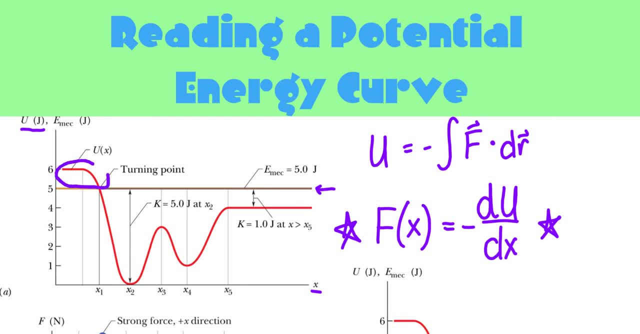 you'll see that this portion before X one on my graph is above this total mechanical energy line. That tells me that the object can never actually reach any location that's to the left of X one, because it doesn't have enough energy. A force would have to do work on my particle or on my 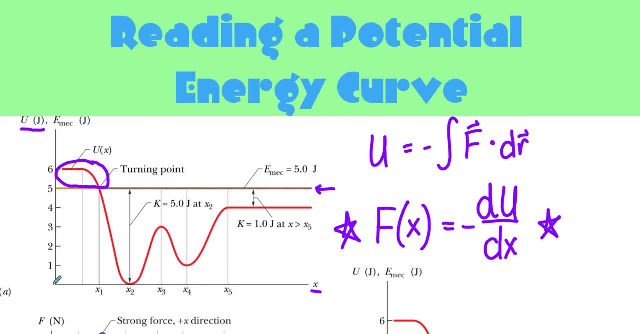 object to get it up. these values get it up anywhere to the left of X one. I can also take a look at X one And I can also take a look at any of these objects And if I have a force, that's other values, and know how much kinetic energy my object has, because mechanical energy is the sum. 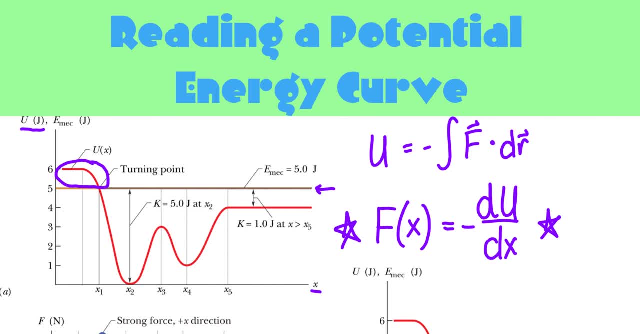 of kinetic and potential energies. You'll see that marked on the graph quite a bit. So for example, at x2 the potential energy is zero. so that means all of its energy is kinetic energy. See, as you see right here. Or for example, at x5 or any location to the right of x5, the potential energy is four. 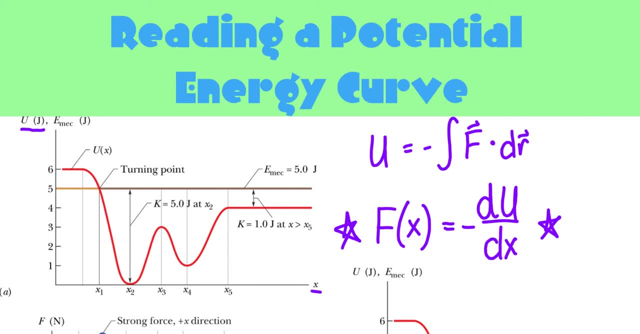 You'll also notice something that's commonly included on a potential energy curve is a straight line that tells us about the total mechanical energy of our object. like you see here, We know that an object's total mechanical energy is a set value. It can never magically. 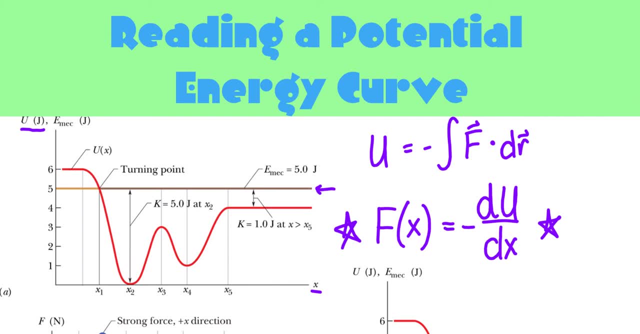 gain energy, and if all the forces acting on it are conservative, it can never lose energy either. So taking a look at where this total mechanical energy is, we can see that the force is acting on the energy curve. and if the force is acting, 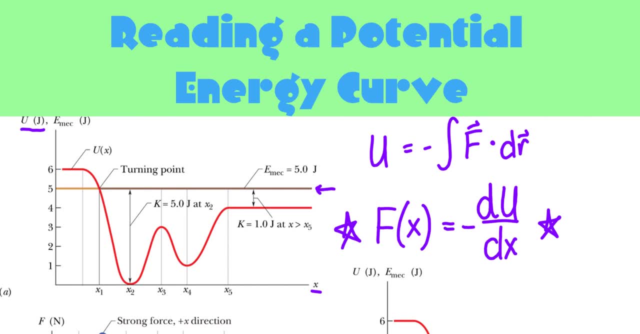 on the energy line corresponds with the graph of my potential energy. it helps me know some things about the motion. For example, you'll see that this portion before x1 on my graph is above this total mechanical energy line. That tells me that the object can never actually reach. 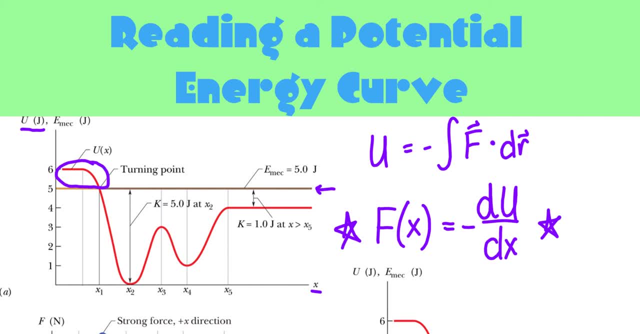 any location that's to the left of x1, because it doesn't have enough energy. A force would have to do work on my particle or on my object to get it up. these values get it up anywhere to the left of x1. So if I have a force that's to the left of x1, and I have a force that's to the left of x1,, 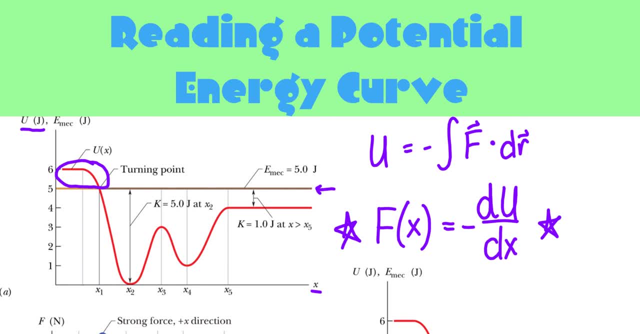 I can also take a look at any of these other values and know how much kinetic energy my object has, because mechanical energy is the sum of kinetic and potential energies. You'll see that marked on the graph quite a bit. So for example, at x2, the potential energy is zero. so that means 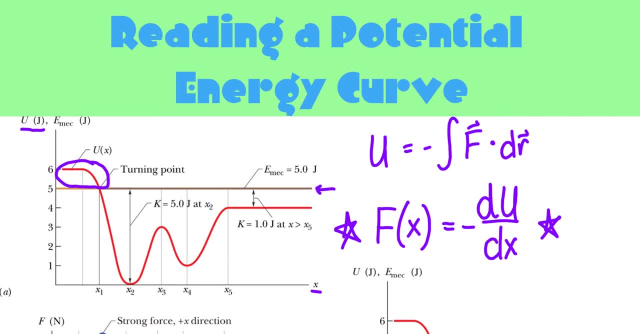 all of its energy is kinetic energy. as you see right here, Or for example, at x5, or any location to the right of x5,, the potential energy is zero. so that means all of its energy is kinetic energy. Or for example, at x6, the potential energy is four joules, which means it must have one joule of. 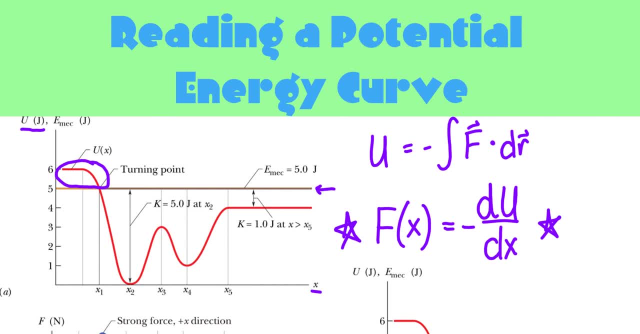 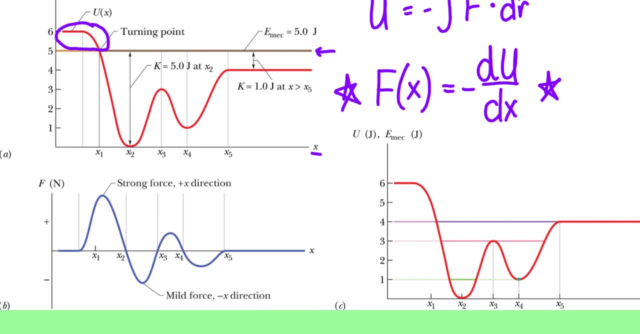 kinetic energy, A couple of other important things about these potential energy curves. We'll take a look at a couple of different examples of these. So any time that you have a turning point, a point where an object changes going from one direction to another, that would be a point where your 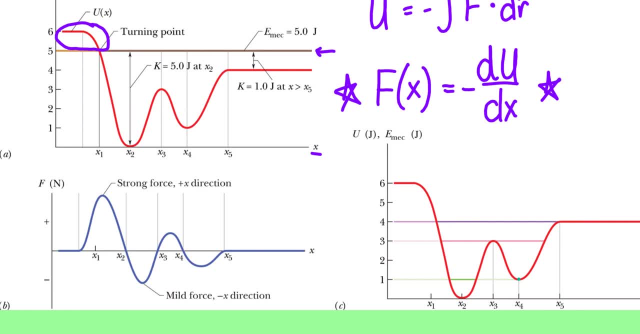 potential energy curve intersects with your total mechanical energy line. We know that because at that point there's no potential energy curve. So we know that because at that point there's no kinetic energy. So all of its energy is potential energy, which means it's not moving and that 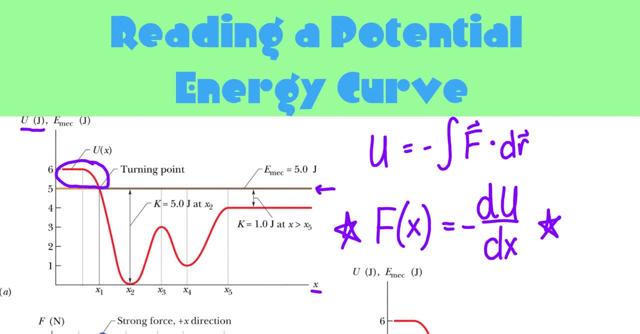 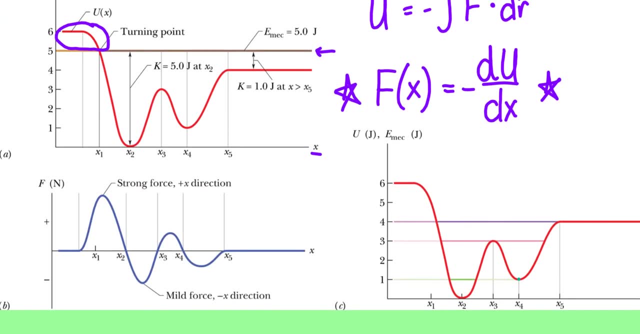 joules, which means it must have one joule of kinetic energy. A couple of other important things about these potential energy curves. We'll take a look at a couple of different examples of these, So anytime that you have a turning point, a point where an object changes going from one, 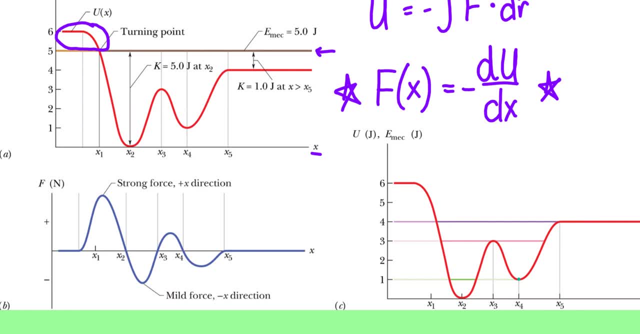 direction to another. that would be a point where your potential energy curve intersects with your total mechanical energy line. We know that because at that point there's no kinetic energy, so all of its energy is potential energy, which means it's not moving, and that corresponds to a